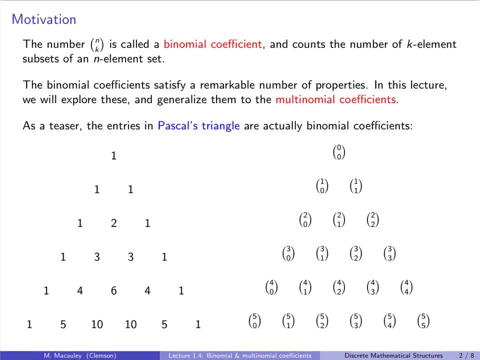 The entries in this triangle are just the binomial coefficients, So some of these are easy to check. All of these entries, n, choose, n- is just equal to one, And I should say that if you call this first row the zeroth row and these entries the zeroth entries in each row, 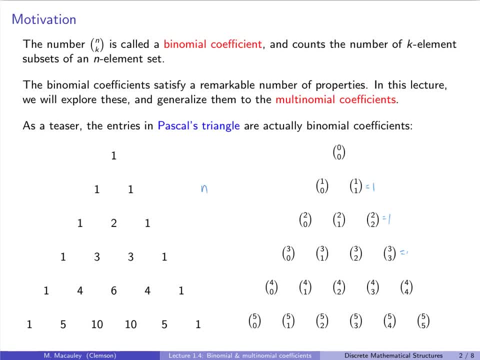 then in row n, the kth entry is n choose k. So we can see why n choose n equals one. There's one way to choose n things from a set of size n, And similarly, there's one way to choose nothing from a set of size n. 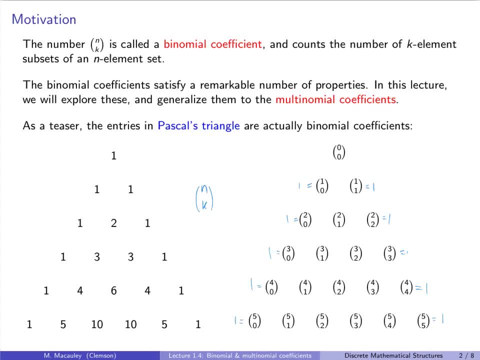 So the outer ones hold. and similarly, zero choose. zero is one, because there's one way to choose: nothing from an empty set. If you don't believe that zero factorial over zero factorial times, zero factorial is equal to one, because zero factorial is equal to one. 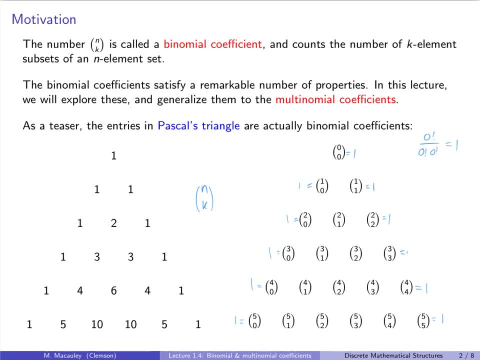 And then, well, you know, to verify this, all you have to do is show that. well, since we have the boundary to show that the remaining thing holds, we just have to show that the same We call this a recurrence relation holds, that each entry is just the sum of the two above it. 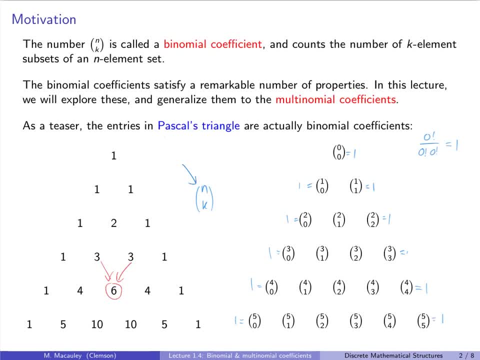 In other words, that n choose k is equal to n minus one choose k minus one plus n minus one choose k. So if we can show that these two things, the sum of these two things, equals n choose k, then it follows immediately that this triangle is exact. 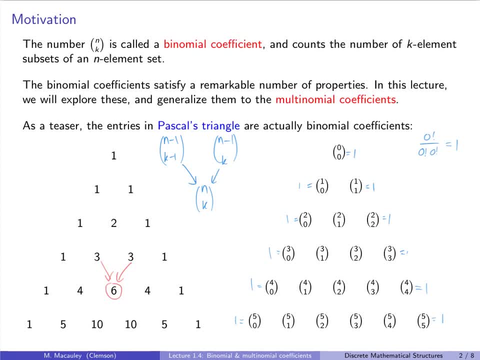 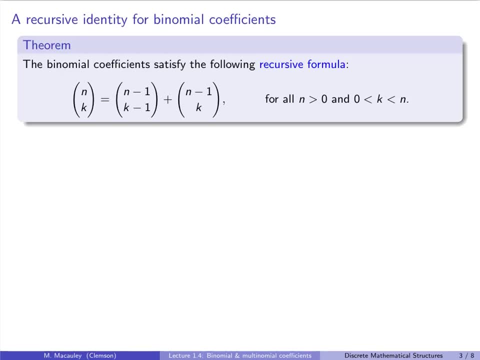 And that's exactly what we want. Okay, so let's do that next. Okay, so here it is formalized as a theorem. The binomial coefficients satisfy the following recursive formula: n choose k equals n minus one. choose k minus one. plus n minus one. choose k. 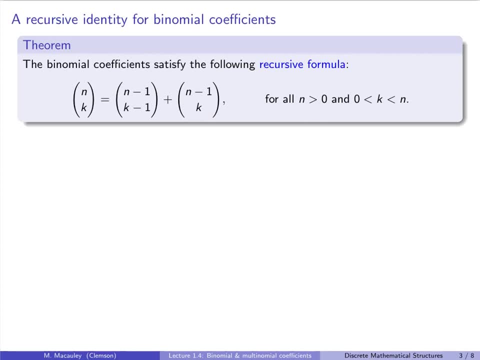 for all positive n and all n between zero, all k between zero and n. So I didn't say that n and k have to be integers, but I think it is clear from the context that that is. that is what is meant. So one way to prove this is algebraically to explicitly show that the left-hand side 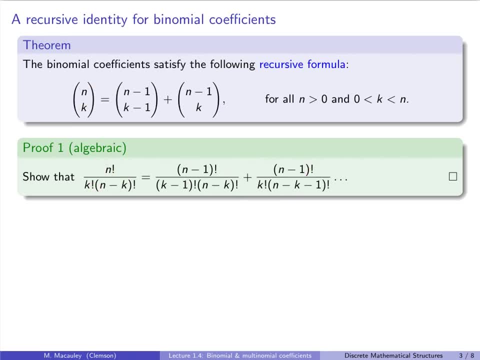 which is this formula is equal to the right-hand side. So how would you show that I'm not going to do it? but I'll give you a hint If you want to add these two fractions. so you somehow want to add these two things and show that they're equal to this. 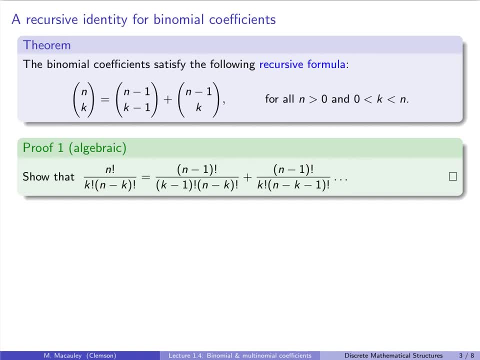 So find a common denominator, And this is almost the common denominator. So to make this the same, if you multiply by k, then this becomes k factorial. And if you multiply this by n minus k, so if you multiply top and bottom by k, 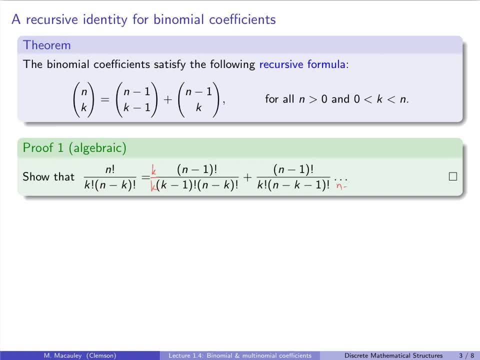 and multiply this by n minus k top and bottom, then this becomes n minus k factorial, And actually this is pretty short. So now the bottom of this is k factorial times, n minus k factorial And the top of this. look what we have. 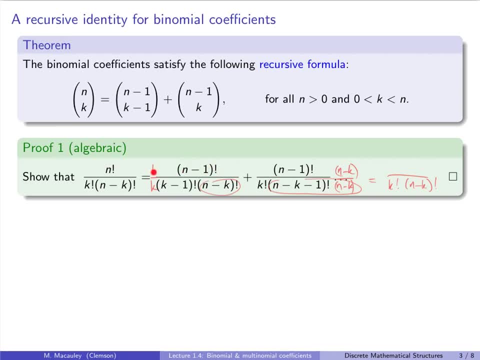 We have. how many n minus 1 factorials do we have? We have k plus n minus k, So that is n times n minus 1 factorial. And look what we have: We have n, so this is just n factorial, which is that. 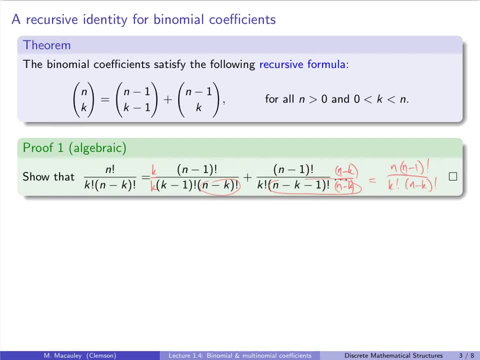 and the bottom is equal to that. So that's one proof. It's pretty short. Here's another way to prove it, Using something that's called a combinatorial proof instead of an algebraic proof. So what we'll do is: 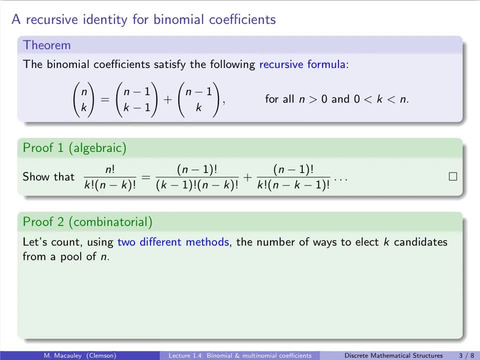 is if we have this identity up here. if we can find something which is counted by the left-hand side and by the right-hand side, then these two things have to be the same. So notice that the left-hand side counts the number of ways. 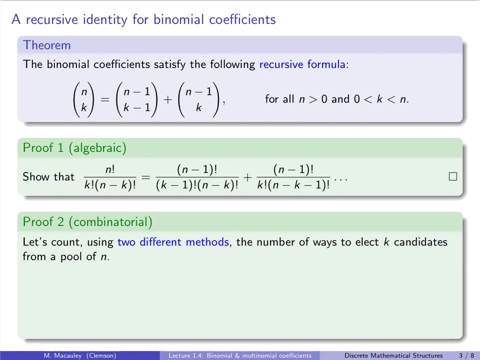 to elect k candidates from a pool of n. So if we can somehow cleverly figure out how to count the same thing using not this formula but this formula, then we know that those formulas have to be the same. So for the second method, the first method is just n, choose k. 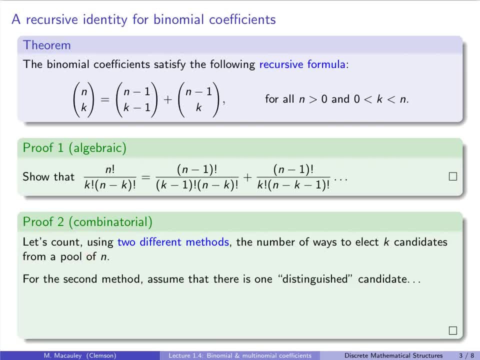 We know how to do that already. Assume that we have n candidates, but one of them is distinct. One of them is special in some way. You can either say special in a good way or special in a bad way. So how many ways? 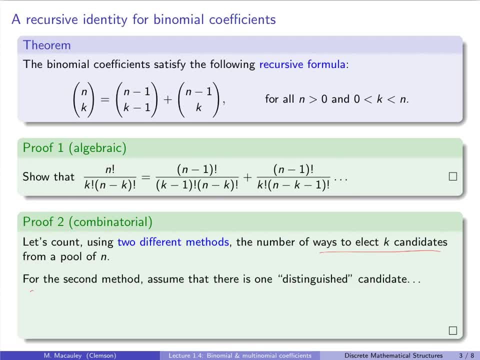 ways do we have to elect k candidates? Well, there's. so there's case one where we, we elect the special candidate to our pool of n. In this case, then there, and then what's what's left? We have k minus one. 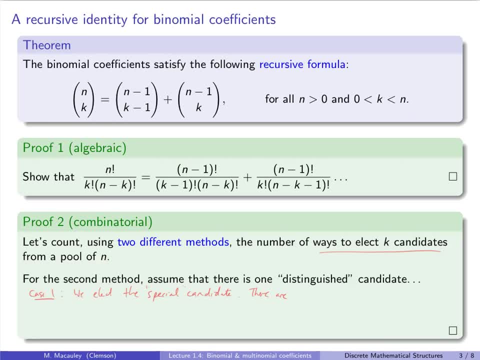 remaining choices. among n minus one choices, Then there are n minus one, k minus one ways to pick the remaining. pick the remaining seats, say. And then case two is we, we don't elect the special candidate In this case, now we still have to elect k candidates, but now our pool is n minus one because we know that we are not including our special candidate. 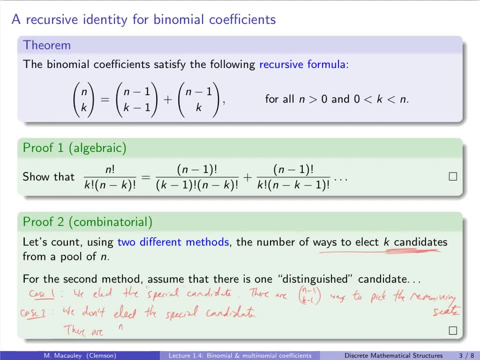 So there are n minus one choose k ways, n minus one choose k ways, n minus one choose k ways to pick or to fill the remaining seats. So all in all, the total number of ways to pick to elect k candidates. 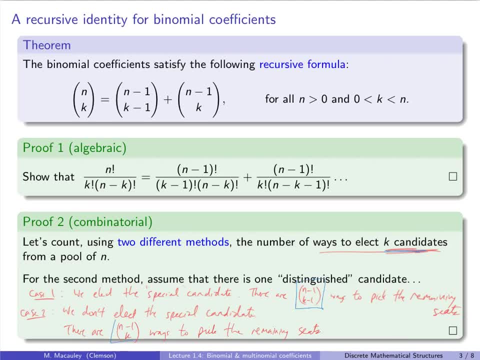 is n minus one- choose k, minus one. plus n minus one- choose k. So so in in in total: n minus one- choose k, minus one, plus n minus one- choose k. So since we have two different ways to count the same, 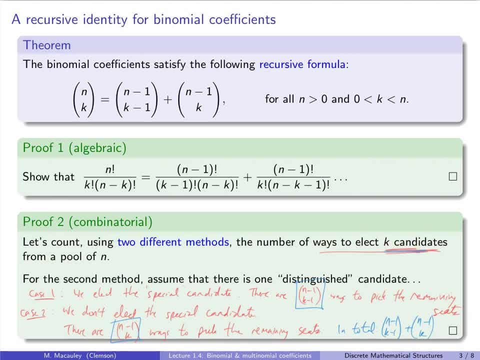 thing, the number of ways to elect k candidates from a pool of n. one of them is just n choose k, which we know and love, and the other one is is is. is this way, then those have to be equal. 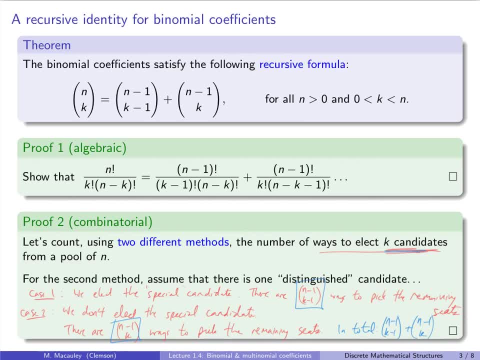 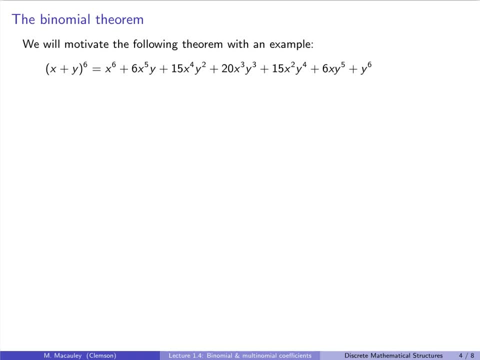 So that's called a combinatorial proof. More on this later. Now we come to something called the binomial theorem, and we will motivate this with an example. Notice that if you take x plus y, two variables raise it to the sixth power. 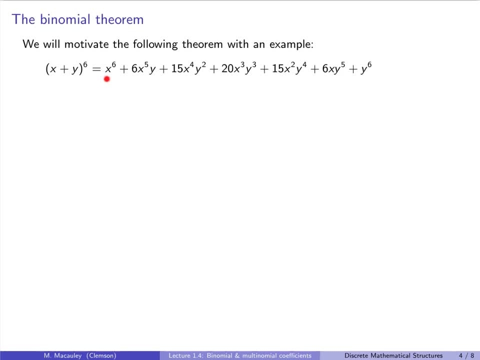 you multiply it out, you get x to the sixth plus six, x to the fifth times, y plus fifteen, x to the fourth, y squared plus twenty, y cubed, x. cubed plus fifteen, x squared y to the fourth plus six, x. y to the fifth plus y to the. 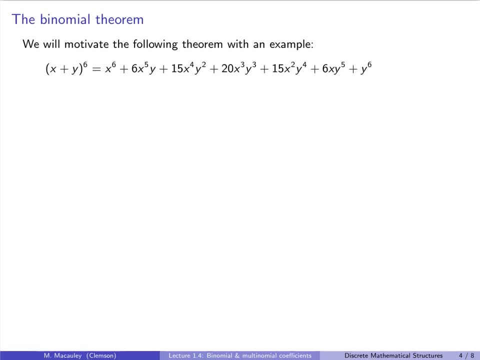 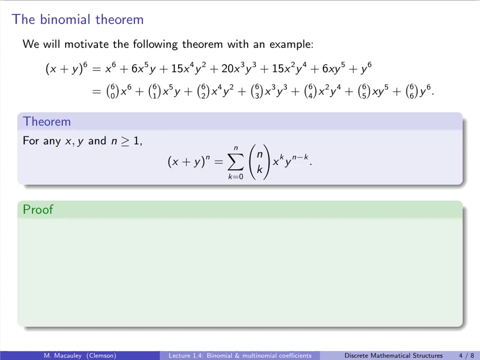 sixth. I'll let you check the details if you want, but let me ask you: do these numbers here, these coefficients look familiar? They might, Because they are binomial coefficients. So let's formalize this. We'll call it a theorem, It's for any. 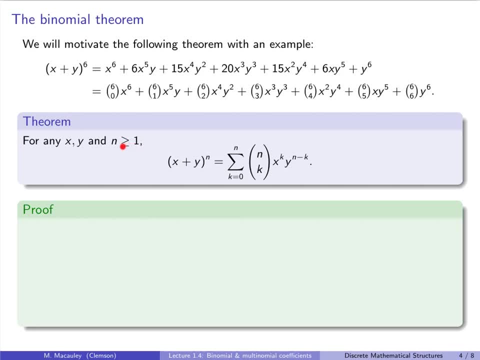 variables x and y and n, at least one, I think it holds, for n equals zero too, but it's pretty trivial, So we'll just focus on this. X plus y to the n. if you multiply this out, you get a whole bunch of. 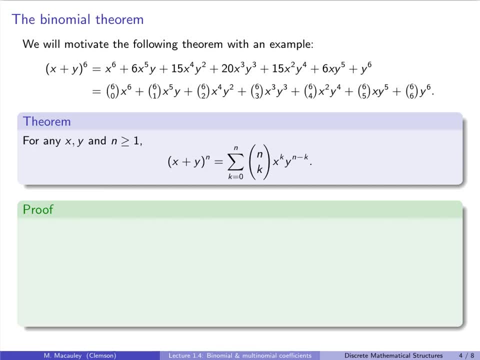 terms and all of those terms. notice that the exponents add up to n, so six plus zero, five plus one, four plus two, three plus three, so forth. So you get a whole bunch of terms of the form, x to the k, y to the n. 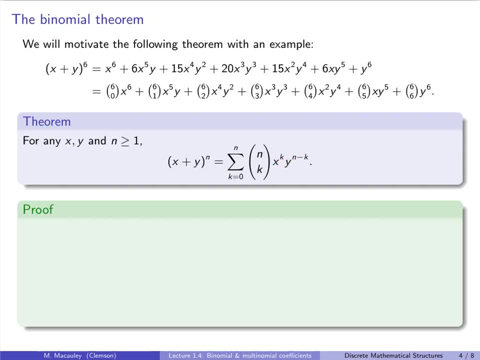 minus k, because these add up to n and the coefficient of this is n choose k. So formally, x plus y to the n is the sum from zero to n of n choose k times x to the k, times y to the n minus. 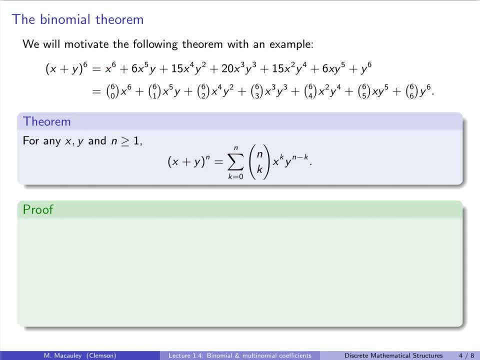 k. So basically it's saying that this thing holds for all n. So this connects this expansion with the rows in Pascal's triangle. It's called the binomial theorem because these are binomial coefficients. Okay, so let's think how we can prove something like this. 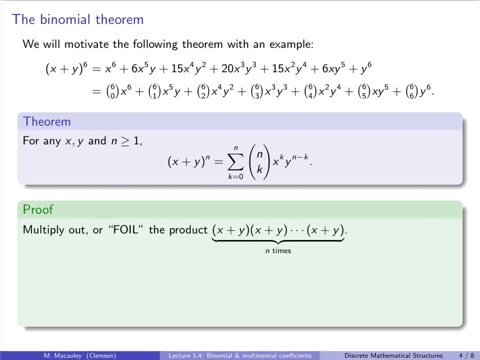 When I say prove, I really mean just verify. Let's start by multiplying out or foiling, remember this acronym. First outer, inner, later, If not all the better, The product x plus y to the n. So here we have. 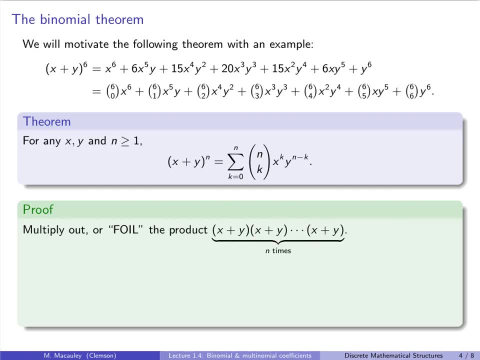 n copies of x plus y, like this, and think about what happens when you multiply this out. So I don't expect you to come up with something like this, but just qualitatively, You get two to the n terms and all of them are going to be distinct. 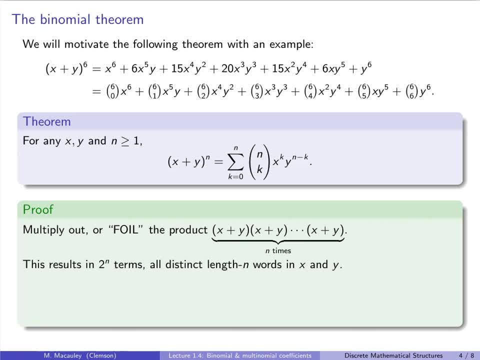 length n words or strings in x and y. I think the easiest way to convince you of this is just to show you For example: for n equals 6, let me write it up here: We get x plus y times x plus y. 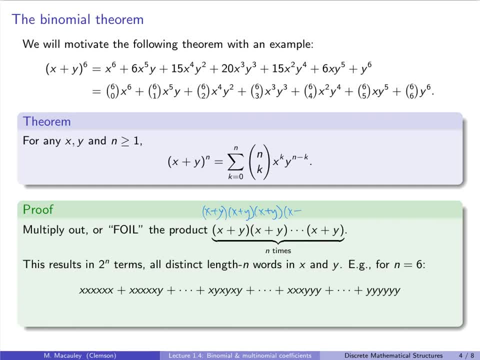 times x plus y- I'm going to do this quickly six times- Here's the fifth one- and x plus 6.. So if we multiply this out, think about how you would do this. You would take this x and multiply it by. 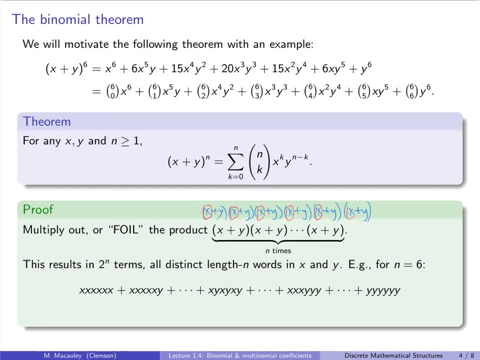 that x times this, x times this, x times this, x times that x, And you get x to the sixth. But you'd also have to multiply by this x times this first five x's and that y. So that's going to get you x to the fifth times y. 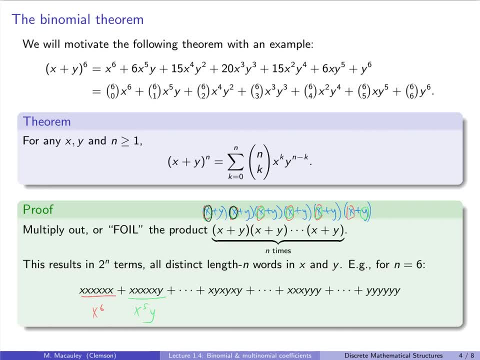 And then you'd also multiply by the first three x's And then the last three y's. So you're going to get a term like that That's going to give you x cubed, y cubed, But you are also going to get an. 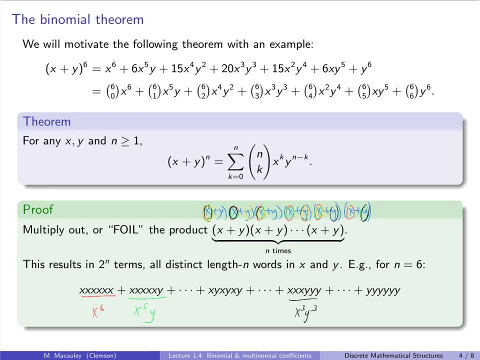 x, y, x, y, x, y. You'll get a term like that. It's going to give you x cubed, y cubed, And you're going to end up getting two to the n terms Again, one for. 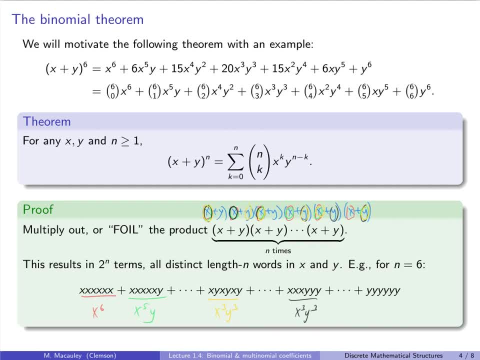 every possible word in x and y, Because you're multiplying one of these two terms times one of these, either an x plus y times an x plus y, times an x plus y, and so forth, And so the coefficient. so if you go out here the 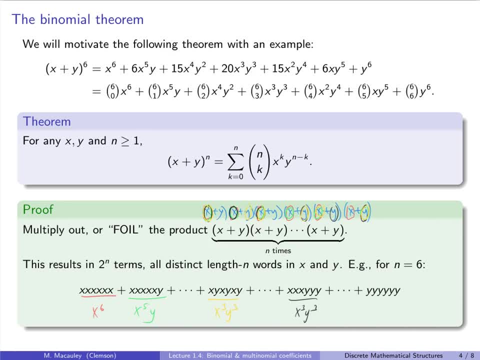 coefficient of say x cubed, y cubed is the number of words in x and y that have length, six words that have three x's and three y's. Now, how many of those are there? Well, it's easier to see if you, instead of x and y's, if you write these as zeros. 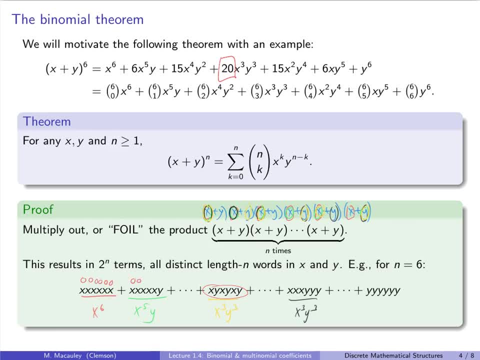 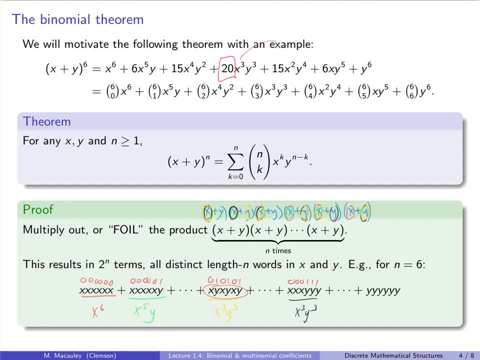 one, one, one. And so now, this coefficient is the number of size, three subsets of a six element set, And we know that that is six choose three. Okay, so to summarize, there are n choose k words with exactly k instances of. 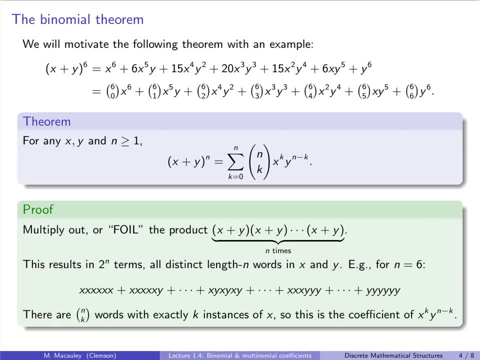 x in. it Easier to see if we're talking about binary strings with k instances of one, And when I say words, I mean length n words where k instances of x and the remaining letters are y. So this is precisely n choose k. 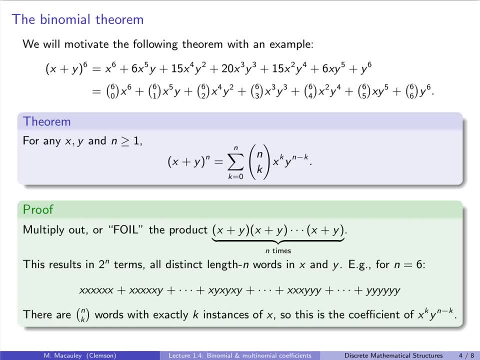 is precisely the coefficient of x to the k times y to the n minus k. Now, one last thing I want to mention is this: identity that we just verified holds for all variables, x and y. So x and y are anything, So we can plug in numbers for these. 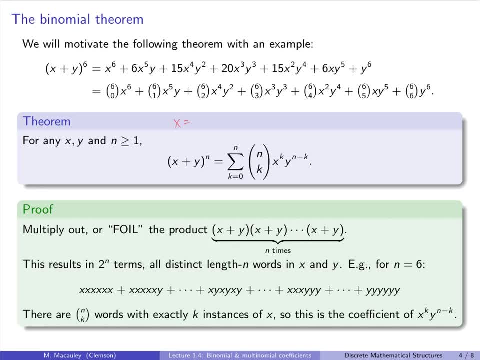 So imagine what happens if you take x equals y equals one. So the left hand side. if we do that is two to the n And the right hand side. these just become one, One to the k times one to the n minus k and we get 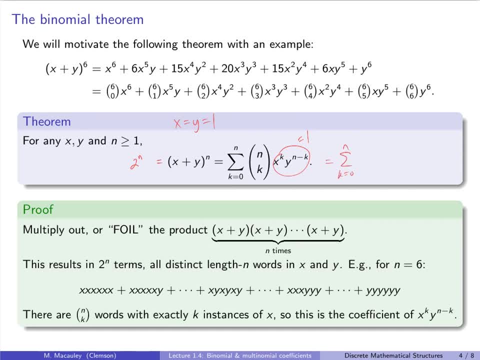 the sum from k equals zero to n of n. choose k. So what that is is that says, if we add up all of these binomial coefficients, in this case we get two to the six, which is sixty-four, And that should be a little bit surprising. 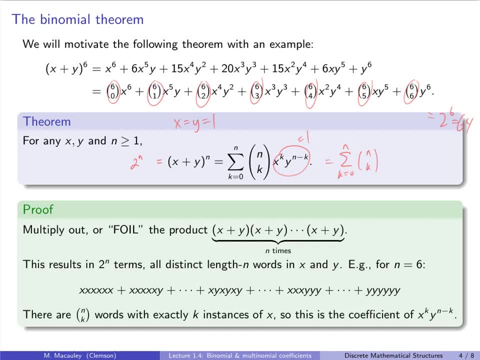 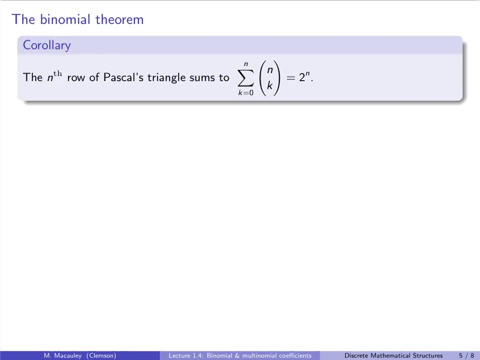 for you. You probably didn't expect that, But if we add up the entries in the nth row of Pascal's triangle, you get two to the n. So this is what we say is a corollary. It's a. it follows from the previous theorem. 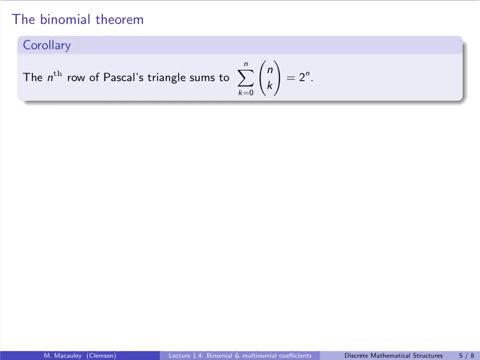 the nth row of Pascal's triangle sums to two, to the n. So remember, if you add up the entries in the nth row, you get n choose zero plus n choose one plus all the way up to n choose n. So the proof of this what I just told you, 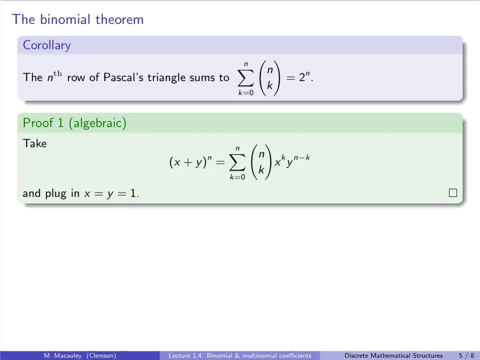 in the previous slide. so here it is written out. just take the binomial theorem and plug in: x and y equals one And, as we saw, it falls right out. So that's one proof. But let me go back and show you a combinatorial proof. 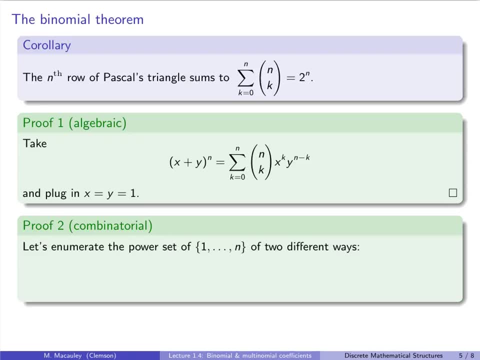 And now recall what a combinatorial proof is. It's a proof that two things are equal, say the left hand side and the right hand side, by showing that they both count the same thing two different ways. So let's. it's not clear how to start. 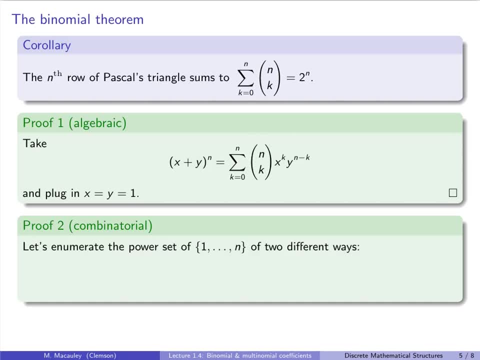 What is going to be counted by this? Well, the left hand side is hard, So let's look at the right hand side. What are things that are counted by two to the n? Well, one thing is the power set of an n element set. So let's try. 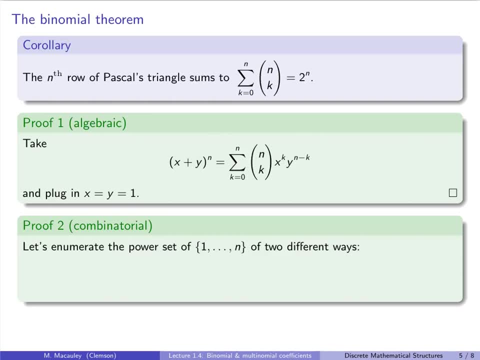 enumerating the power set of an n element set two different ways. The first way: let's just count the number of length n binary strings. This is sort of like what we did earlier. I think I called them true-false questionnaires. 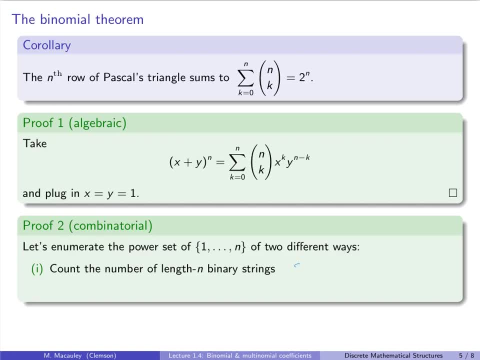 But for example, if you have the subset of, say, n equals six, again, two, three, six, that subset is going to correspond to the binary string zero one one zero, zero one. So this is two, three, six. This is a one in position two, three. 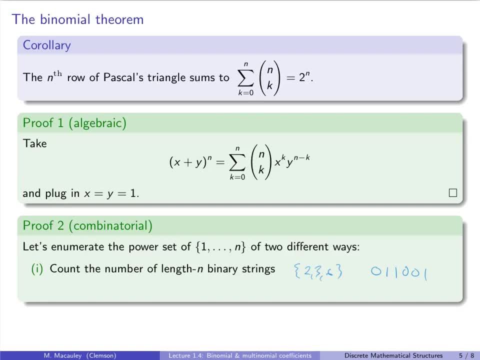 six. Okay, so one way to count the number or one way to enumerate the power set is just count the number of length n binary strings and we clearly get two to the n. And here's another way to count the number of subsets of an n element set. 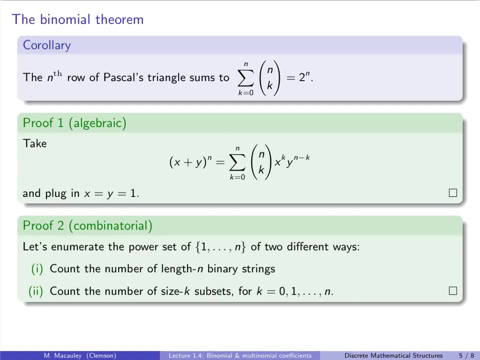 Let's group them by size. So let's first say: how many size zero subsets are there? Well, there's going to be n choose zero Now. how many size one subsets will there be? Well, there's going to be n choose one Now. 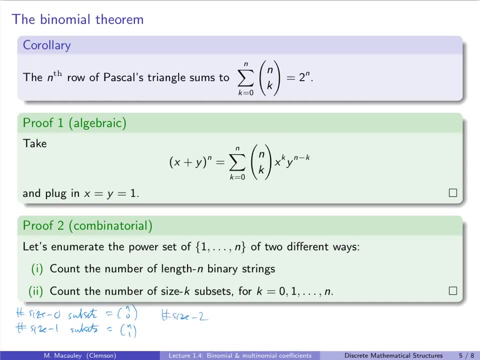 how many size two subsets. Well, there's going to be n choose two All the way up to the number of size n subsets. Oops, I fixed that. That's going to be n choose n. So if you want to add up the number of, 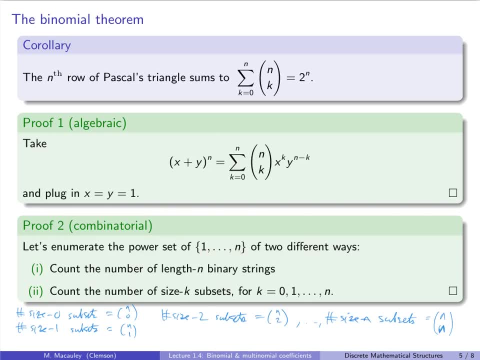 total subsets of this set of an n element set. we can just group them by size. Let's first add up the number of size zero subsets and then add to that the number of size one subsets and add the number of size two subsets all the way up to the number of size. 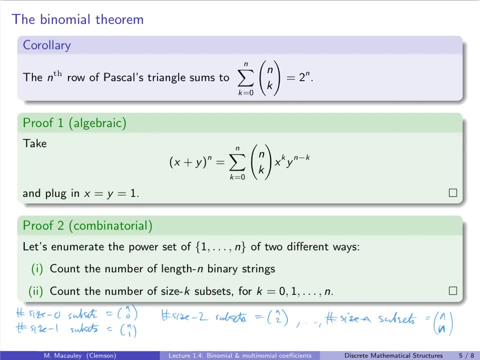 n subsets. And if you do that, what you're doing is you're adding up the binomial coefficients from n choose zero all the way up to n choose n. So that is the left hand side of this equation, And we already know that the number of elements in the 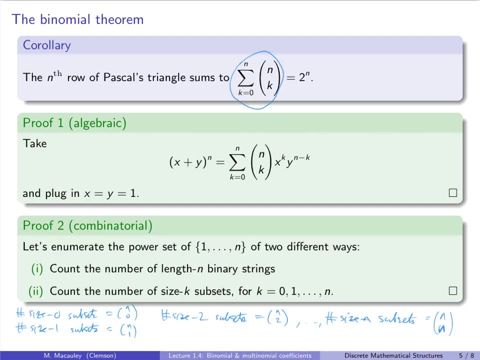 power set of an n element set is the right hand side. So we've counted the same thing- the size of this power set- two different ways. So those things must be equal. So I really like both of these proofs And I'll let it. 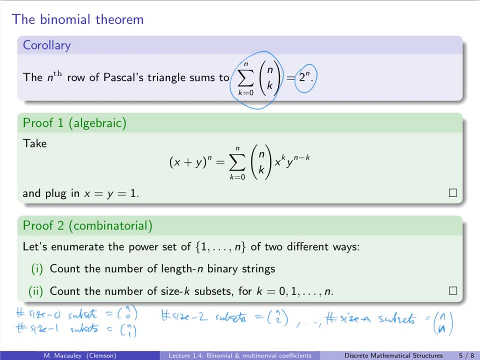 I'll let the choice be up to you as to which one you think takes the cake, Because I think they're both really neat. Let me just finish this slide by reminding you that a proof that establishes an identity by counting a carefully chosen set, two different. 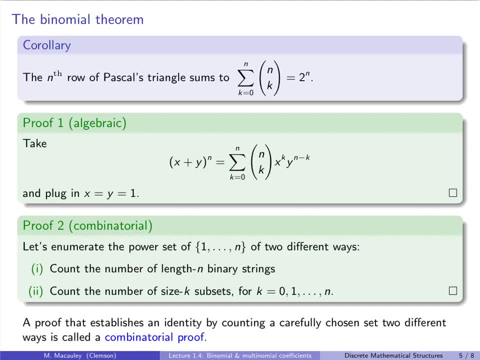 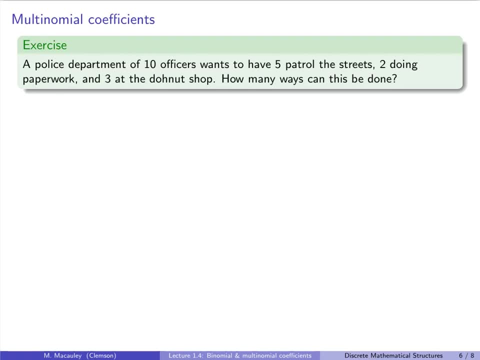 ways is called a combinatorial proof, And more on this later. Our next topic are multinomial coefficients, which are natural generalizations of binomial coefficients. So I will motivate this with an exercise. Consider a police department of ten officers. Suppose that they. 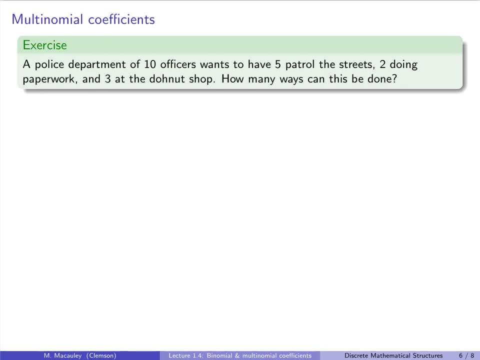 want to have five patrol the streets, two doing paperwork and three at the donut shop. How many ways can this be done? So I'm no longer picking just five from ten, I'm picking five from ten to do one task, two from: 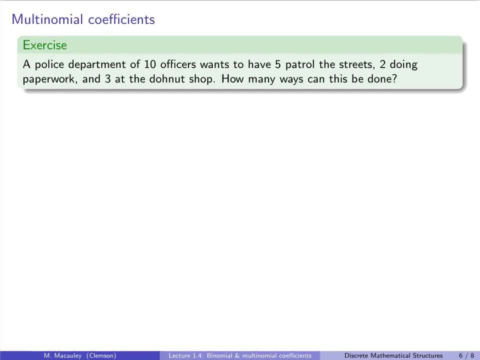 the remaining five to do another task, and then three from the remaining three to do the third task. So to do this, let's see we have ten. choose five ways to pick the five officers to patrol the streets. Then we have ten minus five. 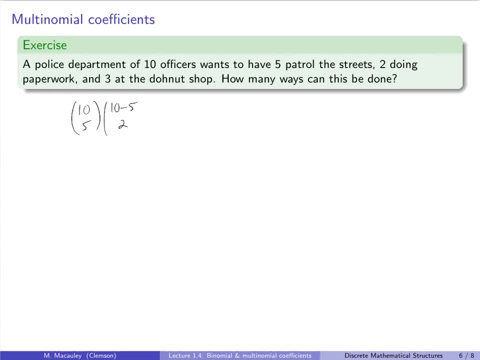 officers remaining and we want to pick two of them to do paperwork, And then we have ten minus five minus two officers left, which is three, and we have to pick three of those three to go to the donut shop. Okay, so the answer to this question 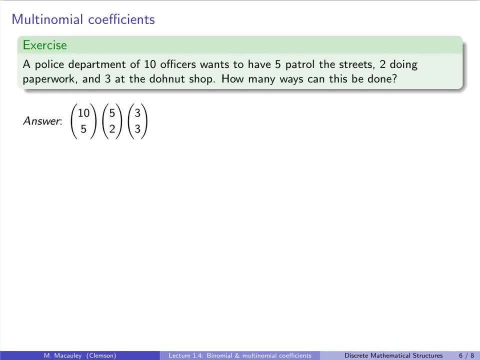 is ten: choose five times five. choose two times three, choose three. Maybe you don't quite see the pattern here as nicely as you did when I wrote it out a few moments ago, But if I multiply this out using factorials, I think you will see a different pattern. 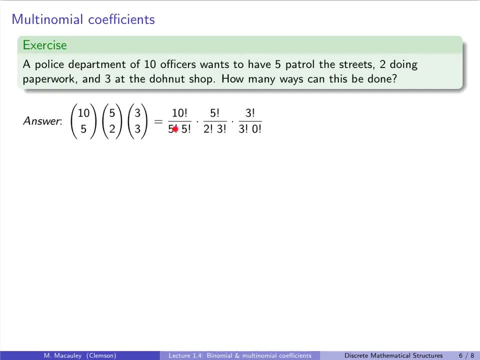 This is ten factorial divided by five factorial times, five factorial times, five factorial. Notice these five factorials cancel Divided by two factorial times, three factorial and that three factorial cancels. with this three factorial Divided by three factorial times, zero factorial. So we get. 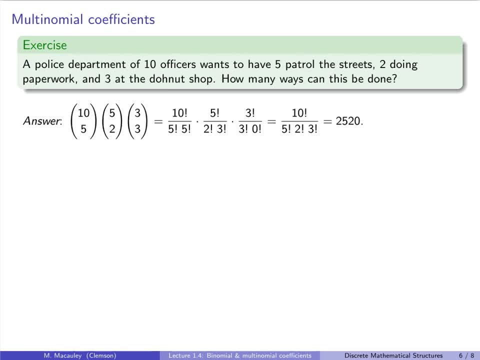 ten factorial, that's the total number of officers. permutations of those divided by five factorial times two factorial times three factorial, which is twenty-five twenty. Note that this is the same as counting the number of distinct permutations of the following ten letter word. 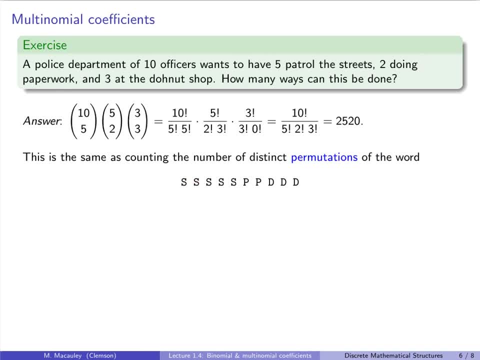 where we have five S's, two P's and three D's. So, for example, this is one permutation, but I can also do: S, P, S, D, D, P, S, S, D P. 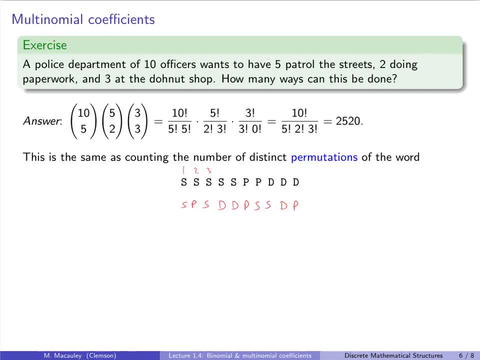 And so think of this as the officers one, two, three, four, five, six, seven, eight, nine, ten, and I am delegating them duties. So this first one says that the first five officers have street duty, the next two 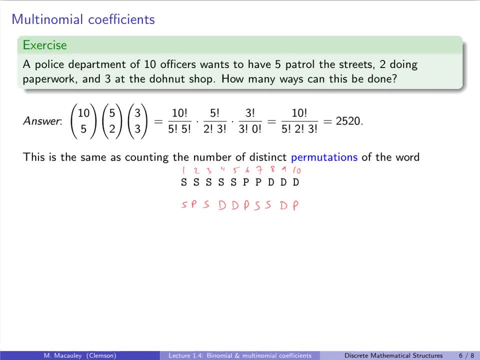 have paperwork duty and the last three go to the donut shop And this one says: officer one does the streets, officer two does the paperwork, officer three does the streets, four goes to the donut shop, and so forth. So the number of 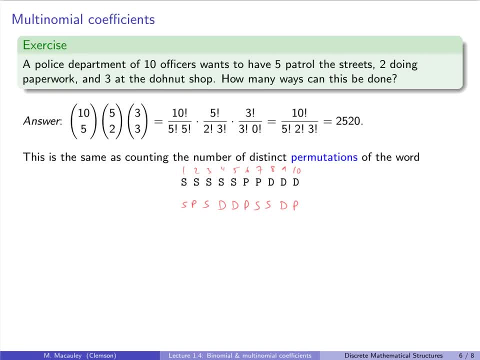 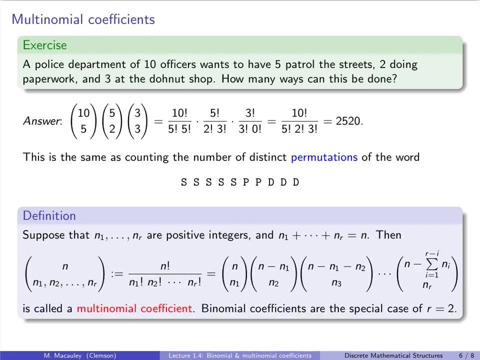 distinct words here that you can form is precisely what we are trying to count. Now that we understand what these things are, let's define them formally. So suppose that N1 up to NR are positive integers that add up to N. Then the following: 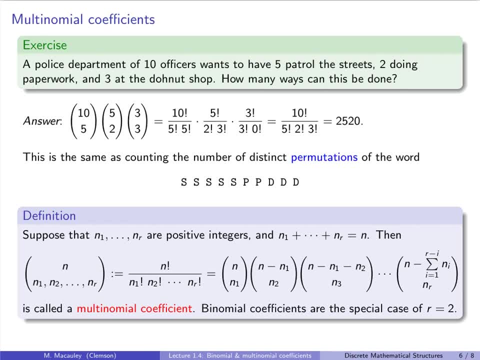 object: it looks like a binomial coefficient. it's got an N up top but on the bottom it's got a list N1 up to NR. I'll skip ahead. that is called a multinomial coefficient And that is equal to. 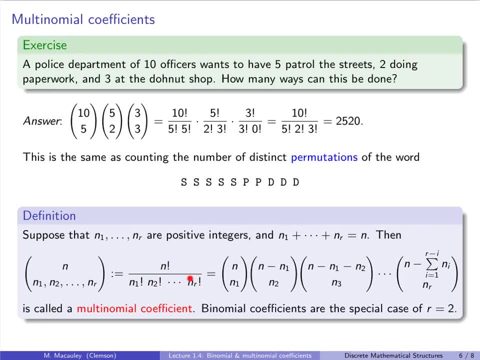 one way to think of it is N factorial divided by the product of N1 factorial times N2 factorial, all the way up to NR factorial, like we did up here. or you can think of it as the product of binomial coefficients N choose N1.. 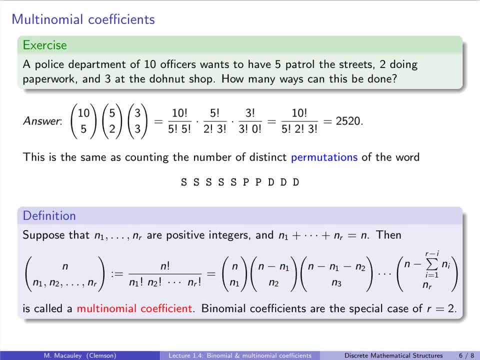 Times N minus N1, choose N2.. Times N minus N1 minus N2, choose N3.. All the way up to N, choose the or N minus the sum of the first R minus I NI's choose NR. Okay, so. 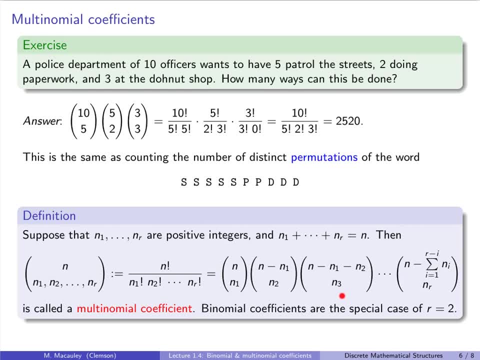 several ways to define it, given. this might be better if you're thinking of officers and this might be better if you're thinking about words. These are called multinomial coefficients and binomial coefficients- notice- are the special case of R equals 2.. 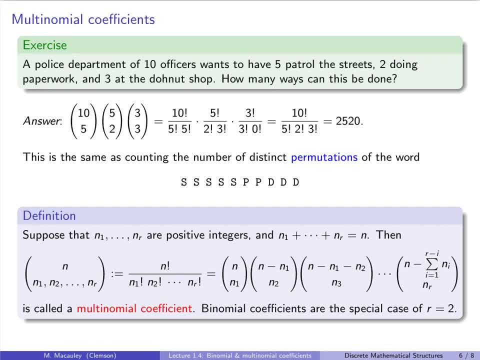 So using this notation, we would actually write a binomial coefficient as N choose K, comma N minus K. but that's kind of silly. there's no reason we would ever do that when we could just instead write N choose K. Let's write down the main points. 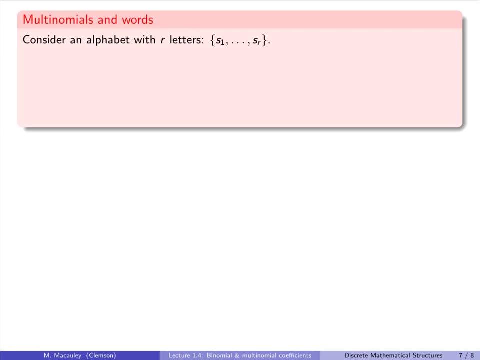 of what we just talked about. Let's consider an alphabet with R letters like S1 up to SR, The number of length, N words or maybe strings. if you're a computer scientist, you can write using exactly N1, S1's. 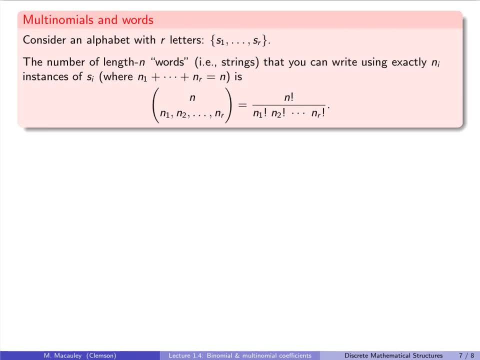 N2, S2's all the way up to NR, SR's. We of course assume that N's add up to N is a multinomial coefficient, so it's N factorial divided by N1 factorial times, N2 factorial all the way up to NR. 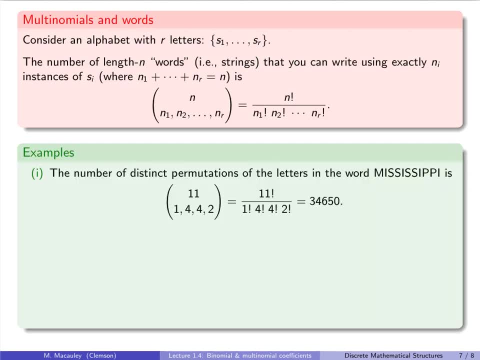 factorial. Let's do some examples. First, the number of distinct permutations of the letters in the word Mississippi, or equivalently words you can form by rearranging these letters or strings. you can form with 1 M, S's, 4 I's and 2 P's. 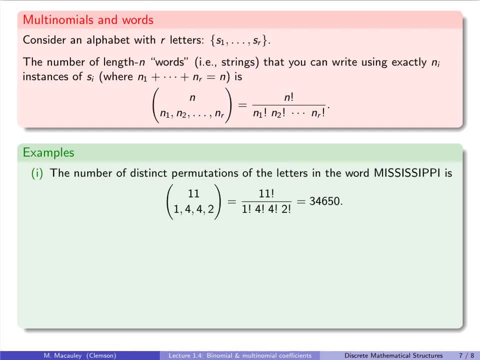 equivalent ways to say the same thing is the following: multinomial coefficient, or just N, factorial over 1 factorial times 4 factorial times 4 factorial times 2 factorial, which is 34,650.. Let me just describe one other way to see this. 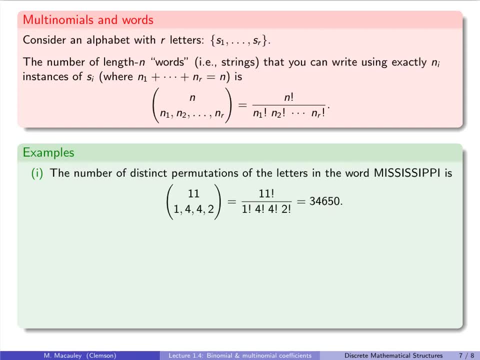 It's nothing new, but it's just something you might like. Another reason why this is true is: let's think of these letters as tiles. What is this? 11 letters. Let's call them M1, I1, S1, S2, I2. 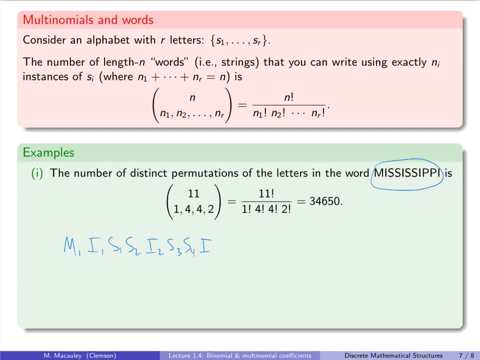 S3, S4, I3, P1, P2, I4. If we actually have these 11 distinct letters, then the number of ways to rearrange them is going to be 11 factorial. However, if at that point, we want to say, okay, let's consider all of the 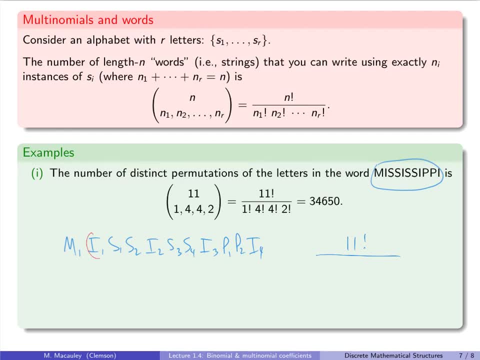 I's the same, then these 4 I's, instead of being so, within the 4 I's, there are 4 factorial ways to rearrange them. so we have to divide, but we're over counting by 4 factorial. Similarly, if we have 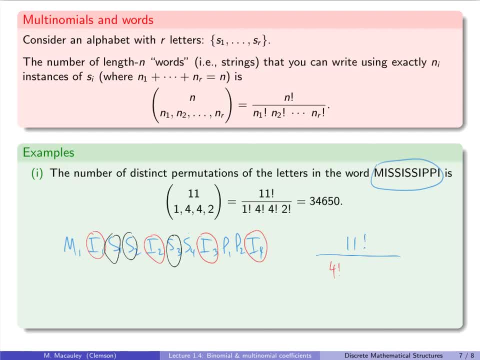 if we want to say that these 4 S's are the same, then there's 4 factorial ways to arrange those that we have to divide out by and same. with these 2 P's, we have to divide by 2, factorial and, of course, 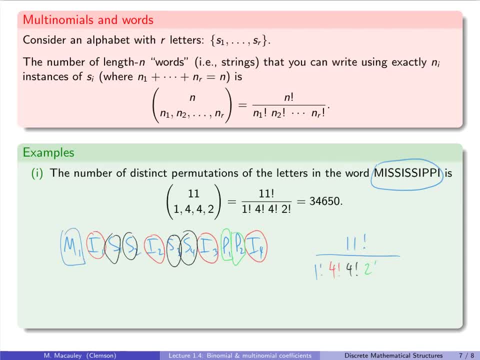 there's this 1 M, which I'm going to leave out here as 1 factorial. So that's just another way to think about why the number of distinct letters in this word is this multinomial coefficient, so you can write this out without even knowing that it is. 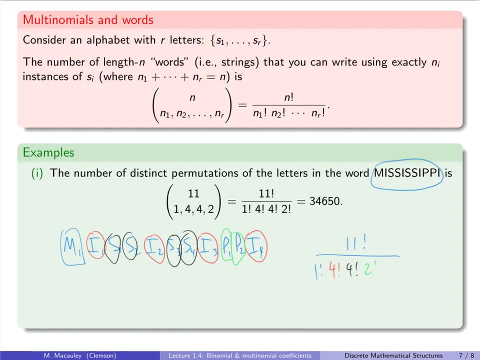 a generalization of a binomial coefficient. So I like this because with this word problem, it was much more natural, I think, to do it this way, whereas the problem with the policeman it was much more natural to do it the way where you have 11. 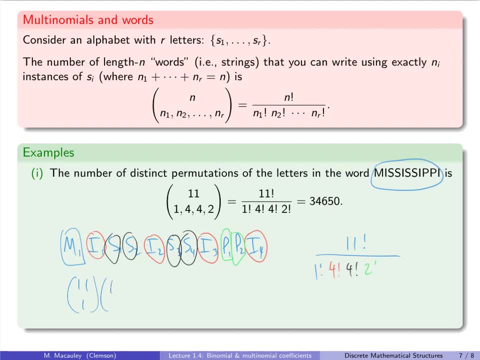 choose 1 times 11 minus 1. choose 4, so you have 1 policeman doing the job that starts with an M machine work. I don't know 4 policemen that get assigned a job that starts with an I ice cream shop. I don't know. 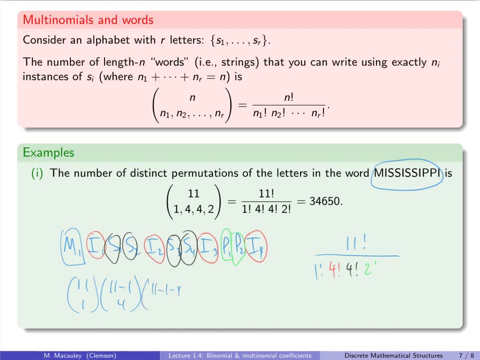 I'm going to just stop. and then 11 minus 1 minus 4- choose 4. that's for the S's. and then 11 minus 1 minus 4, minus 4- choose 2. and of course this is 11- choose 1 times. 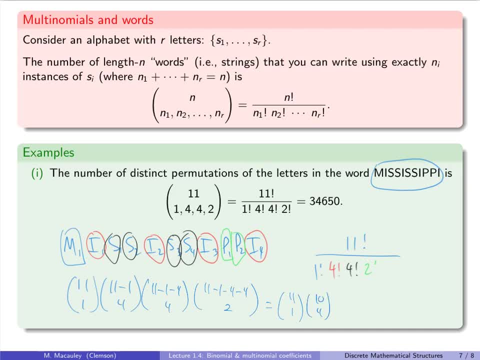 10- choose 4 times 6. choose 4 times 2, choose 2. so to me I don't think it's very natural, when I look at this word problem, to think of it like this. this is a lot more natural, but for the policeman problem. 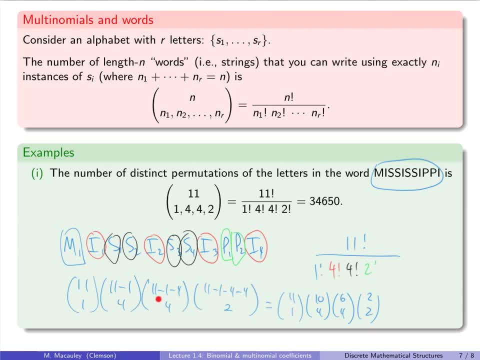 with the donut shop and the paperwork. I think this was the more natural way to do it. when you write out the formulas, you see that things cancel and you get this ok. so two very different ways to think about basically the same type of counting problem. 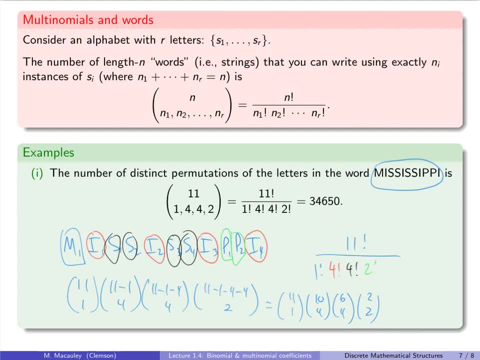 behind the scenes. that's our first example. I want to do one more. it may seem a little bit weird, but there's a reason why I'm doing it, and if you wait until the next lecture on multisets, you'll see why I'm using precisely 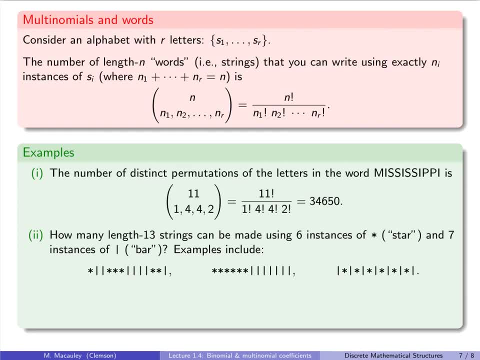 these symbols. our second example is how many length 13 strings can be made using 6 instances of an asterisk or a star and 7 instances of a vertical line or a bar. so examples include star bar bar. star star, star bar bar. star star bar. 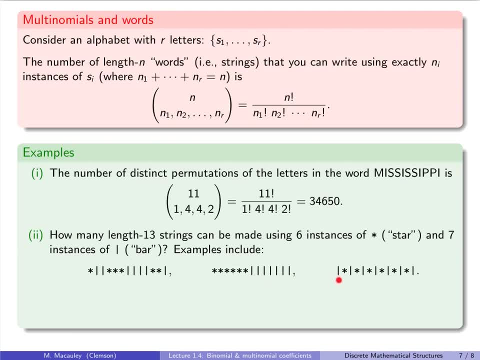 or you can have 6 stars followed by 7 bars, or you can alternate them: bar star, bar star, etc. so I don't know about you, but I learned about this when I was in college in 18, 19, 20, and it didn't strike me as strange. 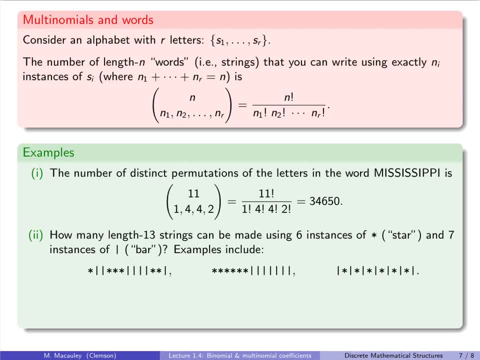 at all the terminology of stars and bars. I went to school in California and then I moved to South Carolina and I started teaching this in my late 30s and I was like wait a second. stars and bars- that is the nickname of the. 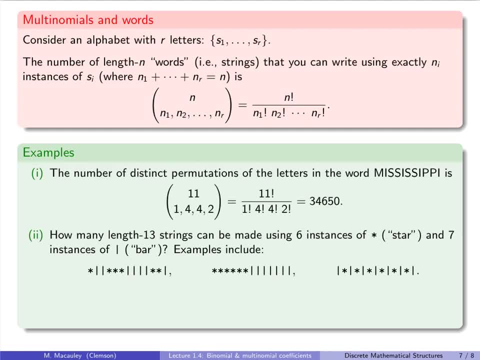 flag of the American Confederacy in the 19th century civil war. this is the pro-slavery part of the US that broke off. now I know I have listeners and viewers of this all over the world who might not know about that part of American history. 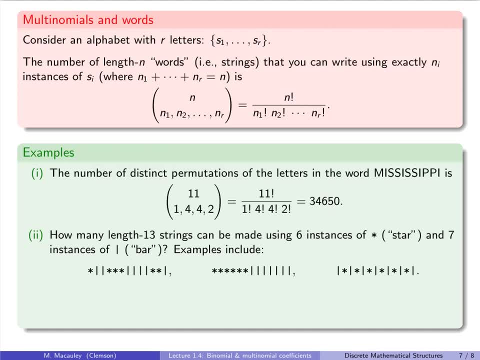 but I certainly was wondering: how did this get this stars and bars, this pro-slavery flag, like? how did that slip through the cracks? and is that just my classroom? so I googled it and no, it is actually a well established combinatorial problem of stars and bars. 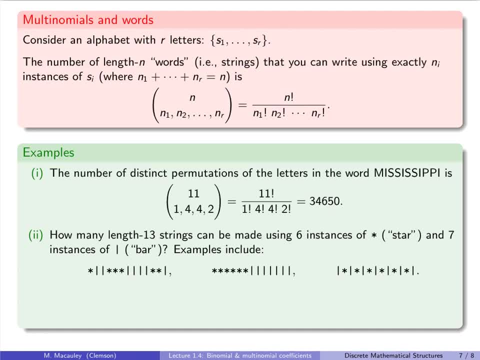 and it dates back to William Feller. if you go to Wikipedia, if you google stars and bars, one of the first things that comes up is combinatorics on Wikipedia and William Feller, who was born in 1906 in the Austro-Hungarian Empire. 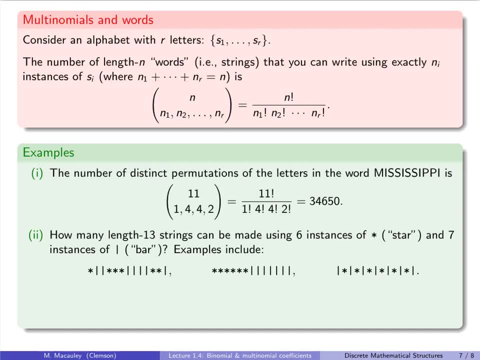 now in Croatia. born in Zagreb, he is the one who came up with this, and the reason for doing it is because this is something that we will see in the next lecture. he wanted something to denote the bars, denote dividers of different regions and the stars. 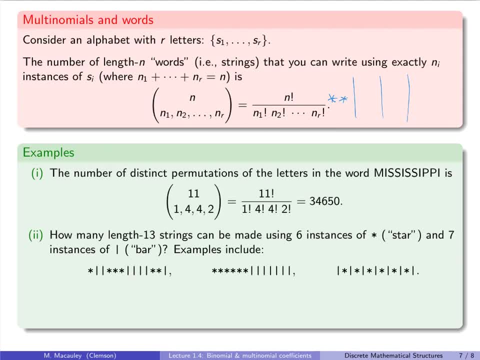 represent different objects, so we will see this next lecture. but suppose you wanted to select things from a vending machine and you have Coke, Sprite water and then, I don't know, Dr Pepper, and you wanted to pick eight drinks so you can pick. so one way to do that is to pick two Cokes. 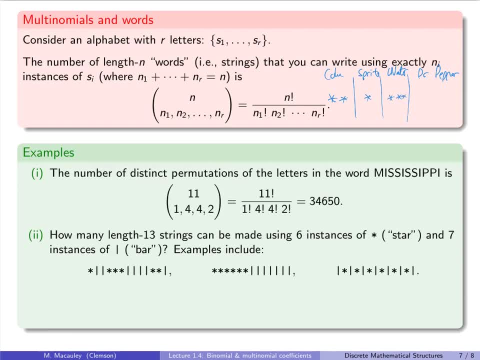 you can pick one Sprite, you can pick three waters and then two Dr Peppers, so you can describe this using a string of stars and bars. so that's where the notation comes from. it's certainly I didn't find it funny the first time I saw it. 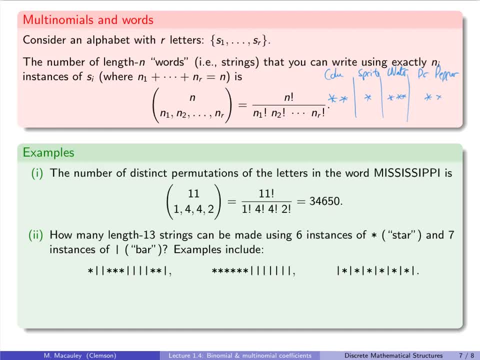 but I did 20 years after that when I started teaching it in the south. ok, so this is something that we know how to do. we know how to count the number of these. the answer is just a multinomial coefficient: 13 factorial divided by 6 factorial. 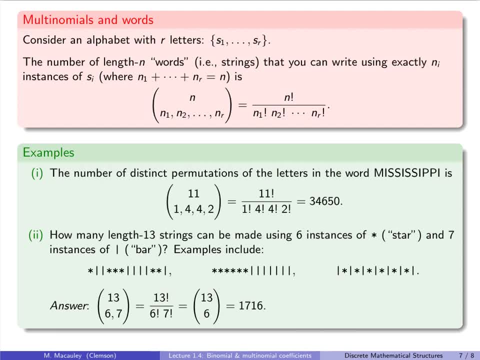 times 7 factorial, which is more commonly known as 13. choose 6 or 1700 and 16. ok. so the reason why I showed this particular example is because we will use this- the stars and bars- in the next lecture when we study. 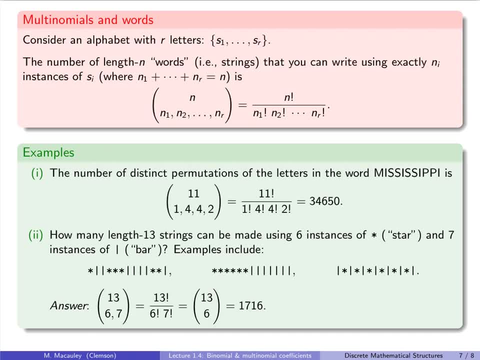 multisets. so this comes up in that so called vending machine problem that I showed you, where you want to pick k objects from n choices but, unlike when you pick k objects from a set of n, you aren't allowed to repeat. when you have a vending machine, you can pick. 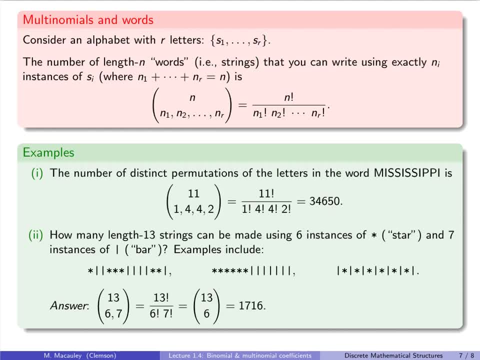 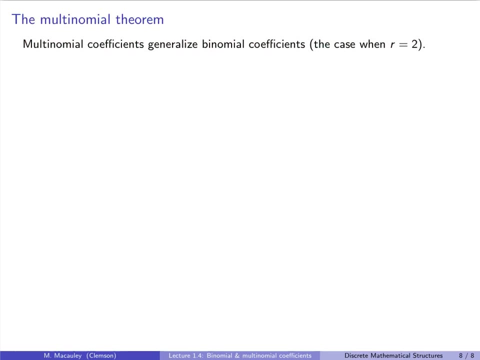 you can repeat, you can pick multiple cokes or multiple sprites. so those are multisets and that will be the topic of the next lecture. but before we do that, I want to have one last word about multinomials, and I want to at least show you the multinomial. 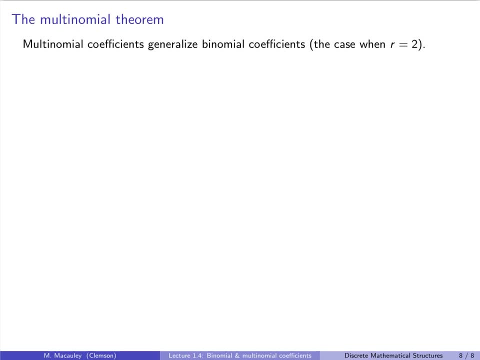 theorem. we're not going to prove it like we did with the binomial theorem, because it's a lot more complicated and really it doesn't come up all that much. so, multinomial coefficients, as I've told you before, they generalize binomial coefficients, which are the special case. 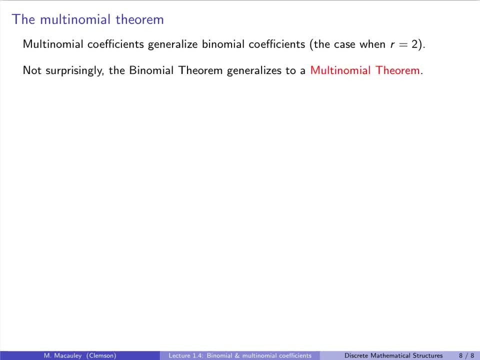 when r equals 2, not surprisingly, the binomial theorem generalizes to a multinomial theorem, and I'm just going to show this to you for completeness or for fun. take your pick. I think it's excellent. it's actually really cool. it's worth seeing. 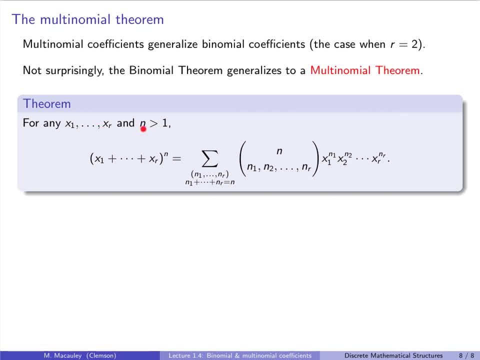 so it says, for any variables x1 up to xr and integer n bigger than 1, if you add up those variables, so x1 plus x2, all the way up to xr, and raise it to the nth power, then you get well, this creature. this is a whole bunch of terms. 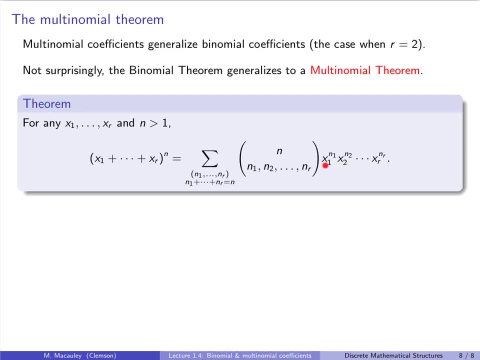 of the form x1 to the products, of the variables x1 to the n1, x2 to the n2, all the way up to xr to the nr, and the coefficient of this monomial is just a multinomial coefficient. n. choose n1, n2. 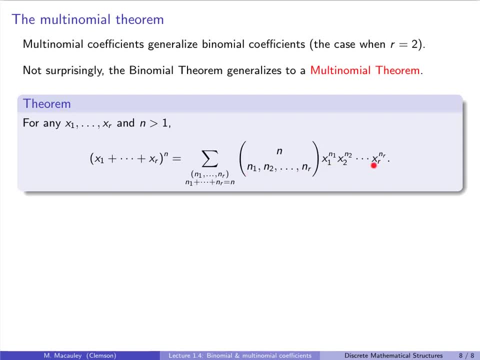 all the way up to nr and we get one of these terms for all possible values of the exponents ni's, where they have to add up to n. so I know this looks complicated, but when we first compare it to the binomial theorem it just says x plus y. 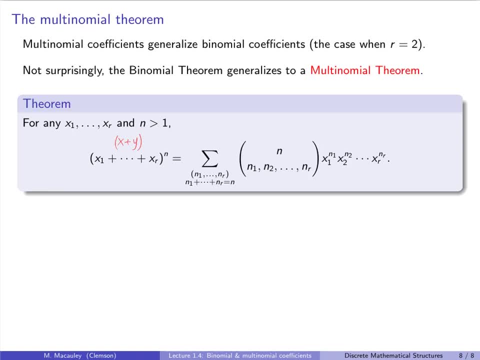 so we don't need. so it's easier to use x and y. if just n equals 2 to the n is just so here we just have x to the k, y to the n minus k. so these things have to add up to the exponents. 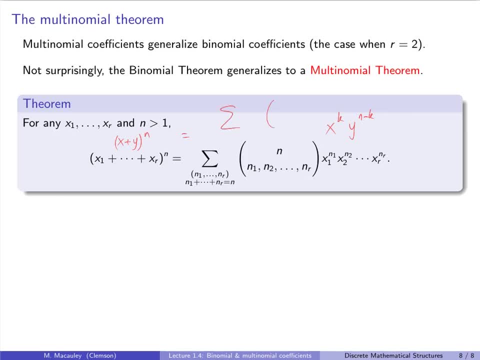 add up to n and then we get the coefficient is the multinomial coefficient: n choose k, comma n minus k, better known as as n choose k. ok, so let's do an example so we can really understand what this is about. so let's do, let's see. 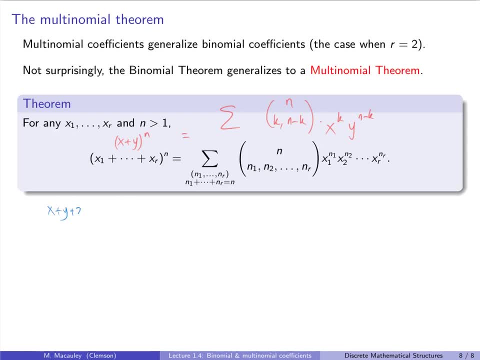 x plus y. I'm going to use x plus y plus z instead of x1, x2 and x3. raise this to the fourth. so all this is saying is that we're going to get a whole bunch of terms that are products of x, so we're going to get an x to the fourth. 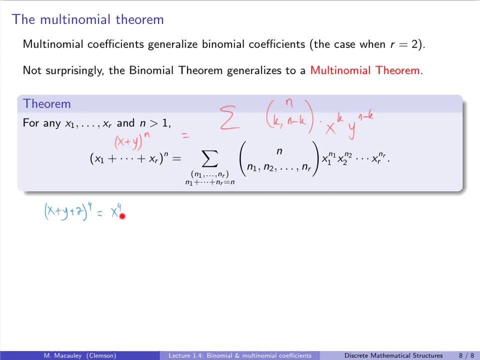 times, I'm not going to write it: y to the zero. z to the zero plus x. cubed times: y plus x. cubed times z plus x. squared times: y squared plus x. squared times: y times z plus x. squared times z squared plus. I hope I'm not missing one of these. 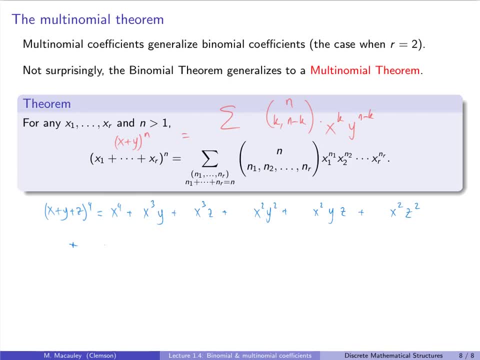 I trust you can catch it if I am x times y cubed plus. so we're going to get- I'm leaving space here because I'm going to fill these in- x times y squared times z. we're going to get some terms of the form y times z squared. 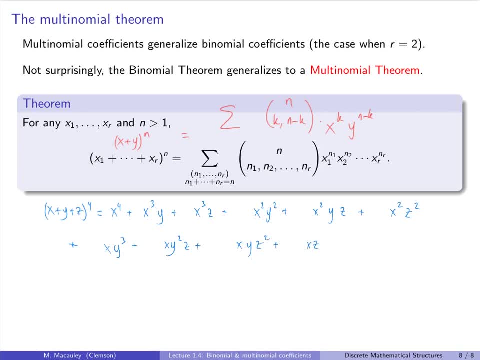 we're going to get some terms of the form x times z, cubed. we're going to get some that are of the form y to the fourth, some that are of the form y, cubed z, some that are of the form y, squared z, squared, some of the form y times z cubed. 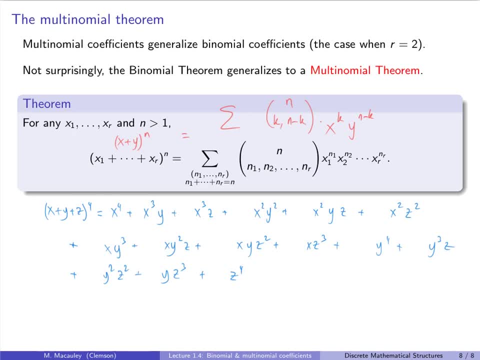 and finally some of of the form y to the fourth, and what this is saying is that the coefficient of each of these, so the coefficient of x to the fourth, is just going to be four choose. I didn't leave myself very much room: four, choose, four comma, zero comma. 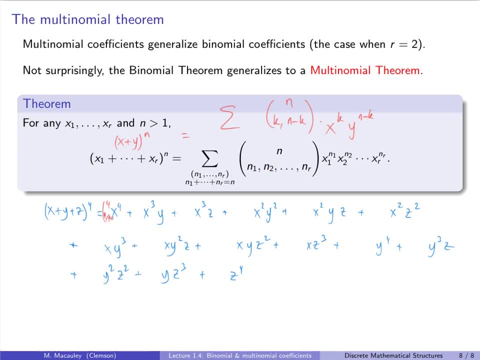 zero. so four comma zero, comma zero. that's just going to be equal to one. similarly- let me just go down, I'm not going to do all of these MNZ- 1 comma 1 comma 2. This is 4. choose 1 comma 2 comma 1. again. I'm just taking the exponents of these things. 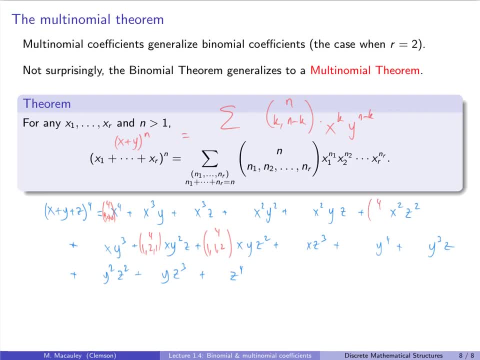 So up here We have 4 comma 2 comma 0 comma 2. Here we have 4 choose 0 comma, 4 comma 0, that's just going to be 1, and I think you get the idea. here We have 4 comma 2, choose 2 comma 1, 1, and so forth.